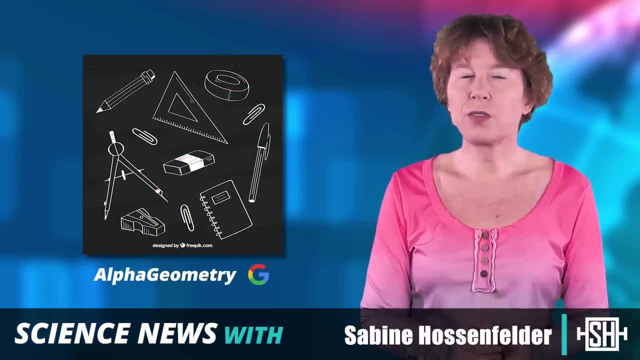 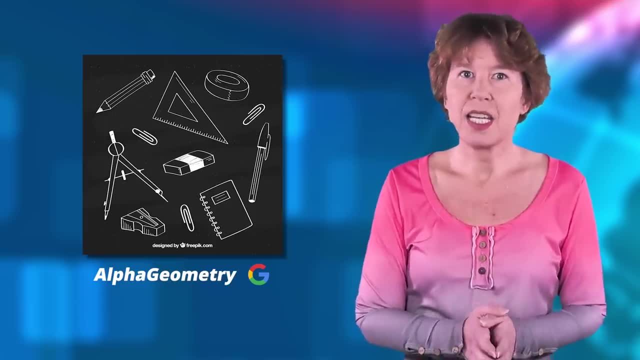 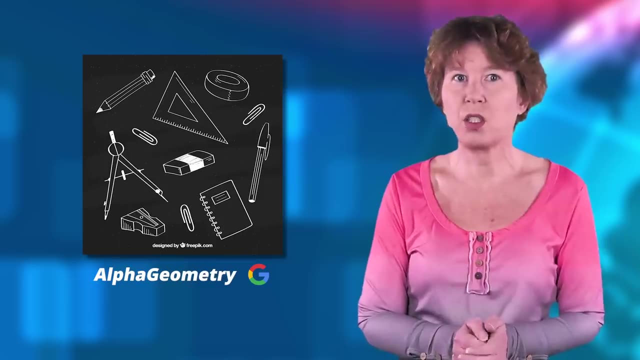 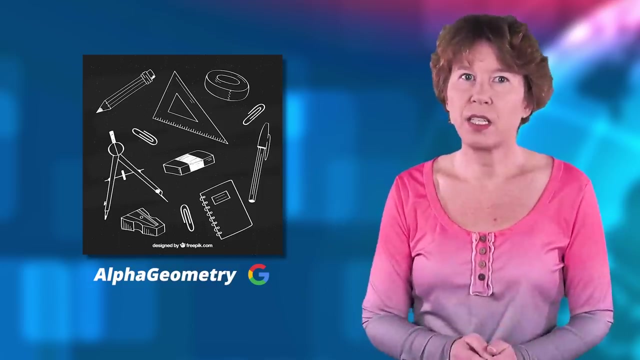 Google has unveiled a new artificially intelligent system, Alpha Geometry, that can solve problems of mathematical geometry. It's the first computer program to surpass the average performance of participants at the International Mathematical Olympiad. That might sound like an incremental improvement. just one more thing that AI is really good at, but mathematics isn't just. 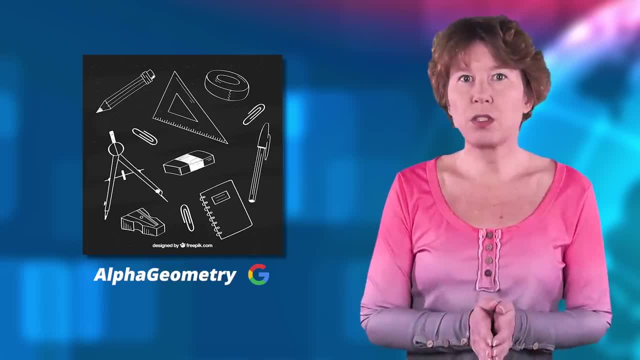 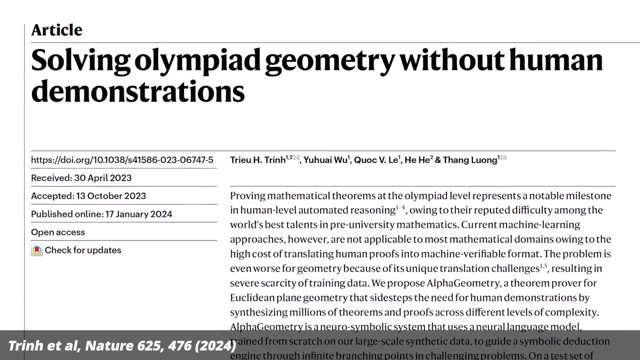 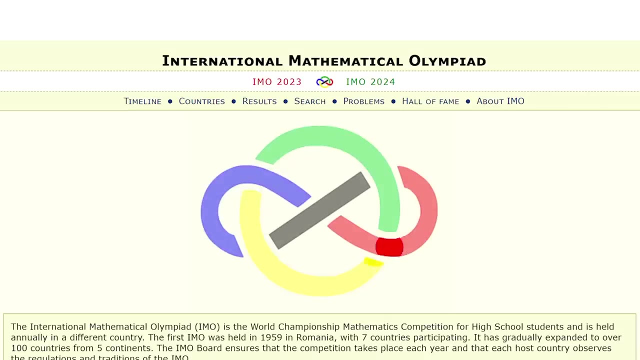 one more thing: it's everywhere. This makes Google's recent development a significant step forward. Let's have a look. This new research was done by scientists at Google DeepMind and Google Research and just published in Nature. They tested their new program, Alpha Geometry, with a set of problems. 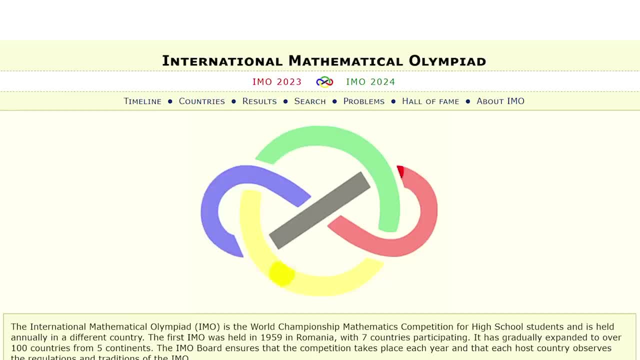 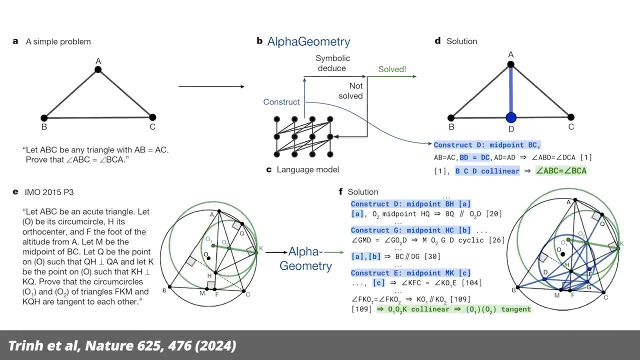 posed at the International Mathematical Olympiad during the years 2000 to 2022.. After the program was trained, it was given 30 Olympiad geometries. The AI solved 25 of them correctly within the standard Olympiad time limit. This performance 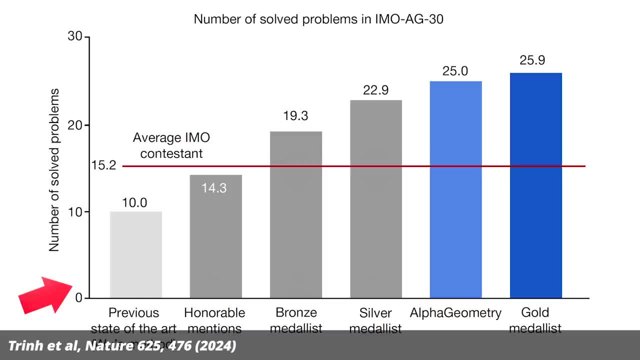 far surpassed the capabilities of the previous state-of-the-art system, which could only solve 10 of these geometry problems. To put this into perspective, the average participant at these Olympiads solves about 15 problems correctly. A gold medalist typically solves. 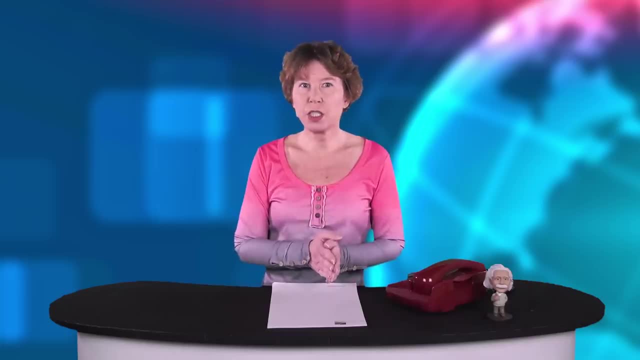 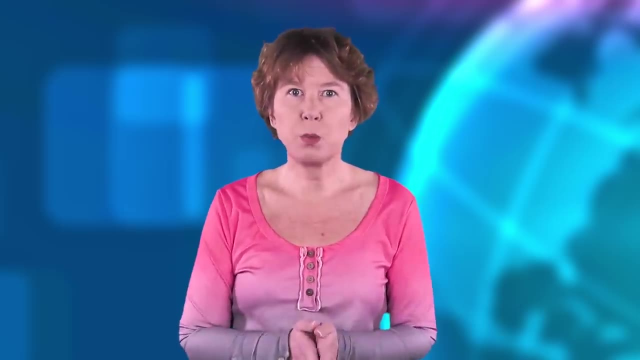 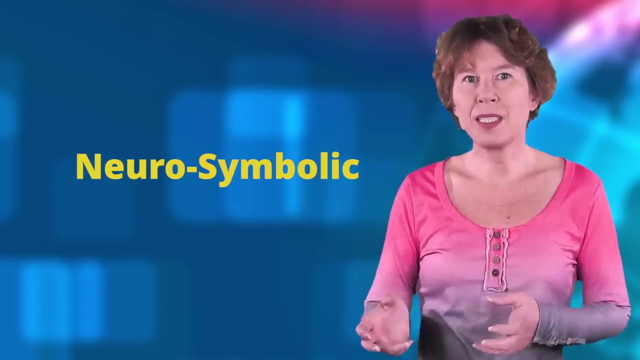 almost 26.. So the new AI is better than the average, but not quite as good. Alpha Geometry uses what's called a neuro-symbolic approach. That means it combines a neural language model like ChatGPT with symbolic deduction like that used by software like. 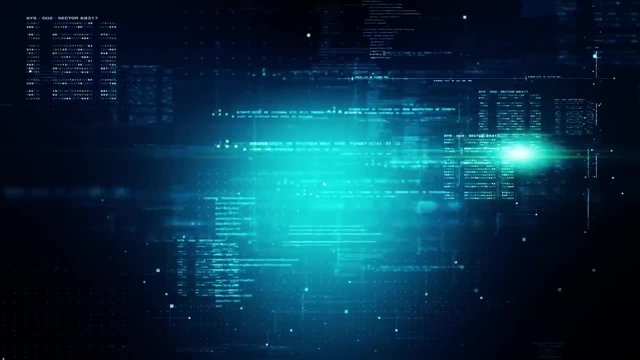 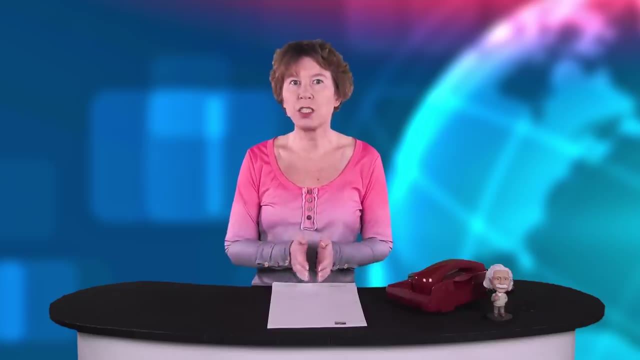 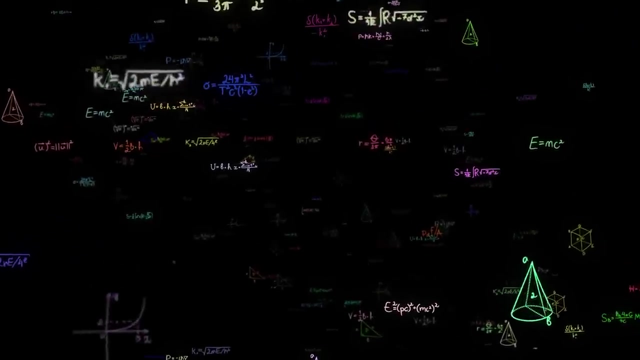 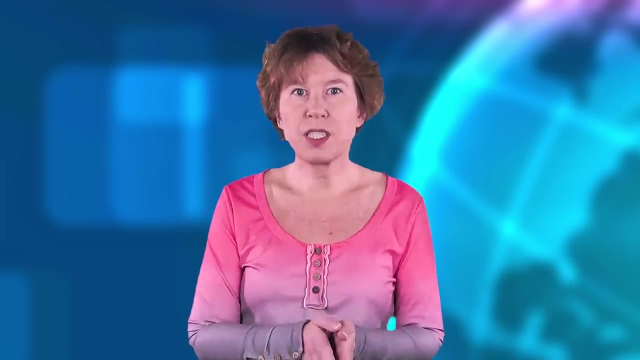 Mathematica. The neural language models are good at identifying general patterns and relationships and data. This makes it possible to quickly come up with potentially useful algorithms. The symbolic deduction programs, on the other hand, basically allow to infer logical relationships. The combination of both makes for a very, very powerful system. It's indeed much more similar. 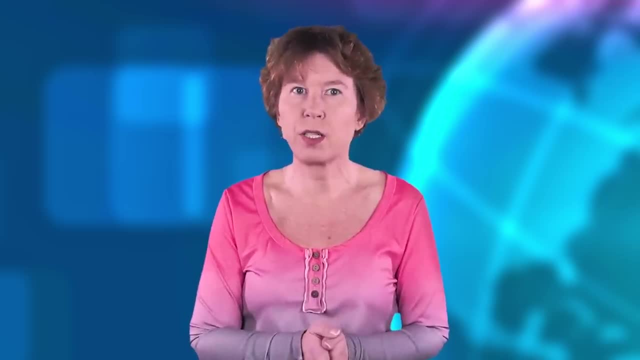 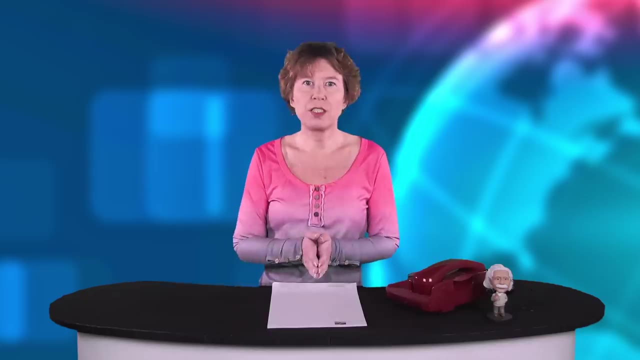 to how the human brain works than just neural networks, because it combines intuitive ideas that we extract from input with more deliberate, rational decision making, similar to Kahneman's System 1 and System 2 thinking. It's a lot more simple to use the neural language model. 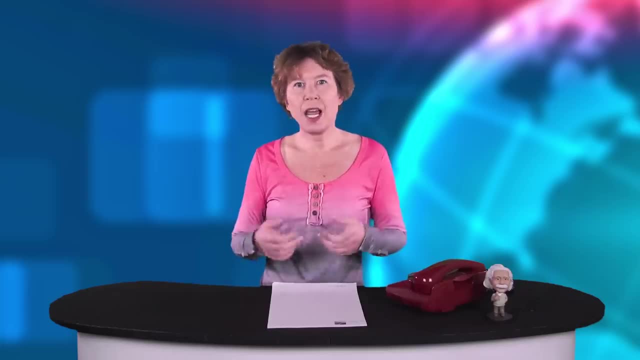 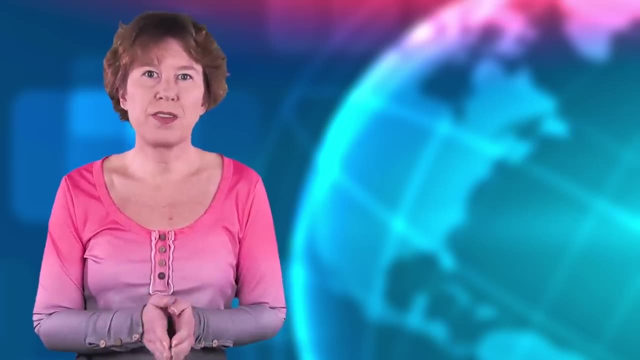 than the neural language model, because the neural networks are the core of the human. It's like, basically, alpha geometry has what chat GPT is missing. it understands logic, One of the problems that have so far prevented AI from becoming good at maths in general. 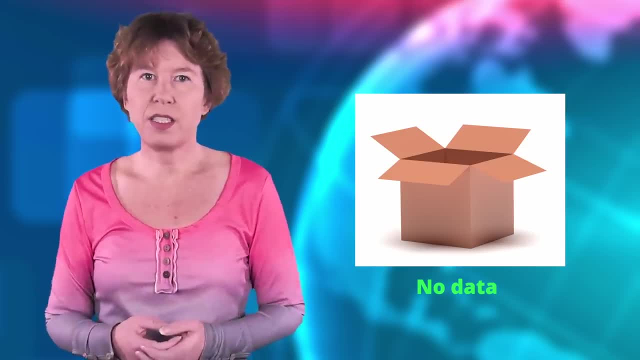 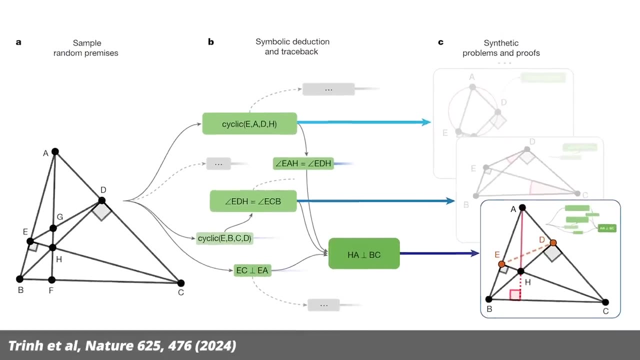 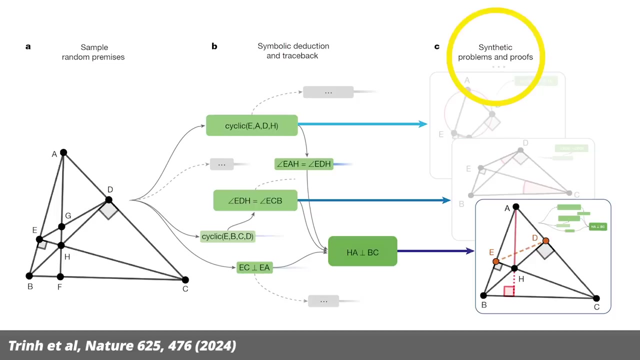 or geometry in particular, is the lack of training data. There are only so many proofs that humans have written down that you can train them on The Google. researchers have addressed this by first generating a vast pool of synthetic proofs that added up to as much as 100 million examples. 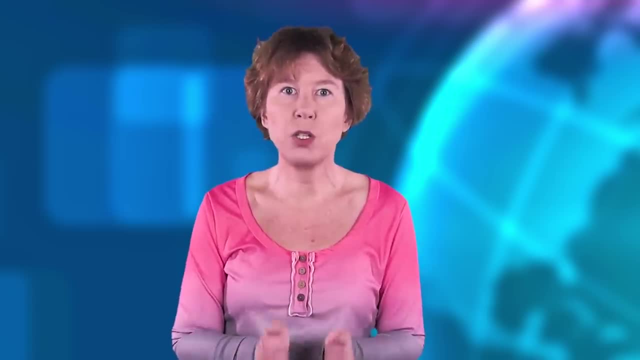 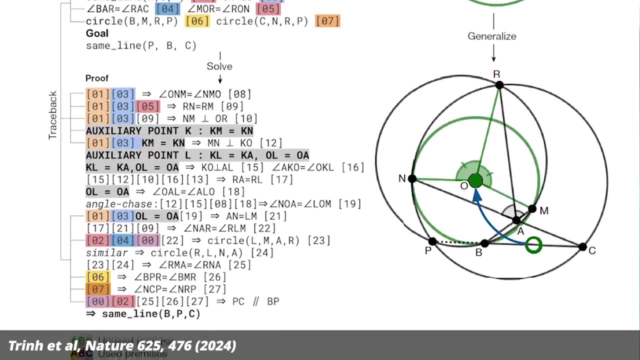 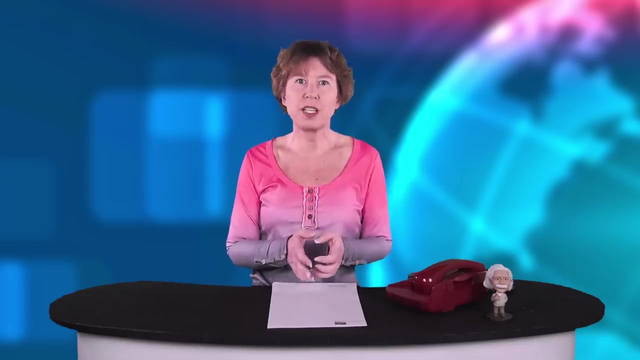 Thanks to this, alpha geometry could train without relying on human demonstrations. Better still, alpha geometry doesn't just spit out a result, it delivers a human-readable, step-by-step proof. Basically, it works by trying to find a sequence of steps that logically fits together and 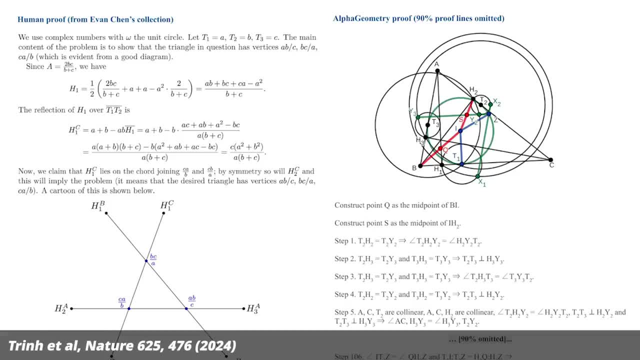 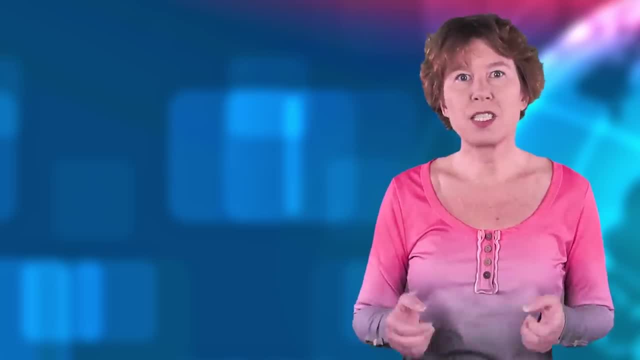 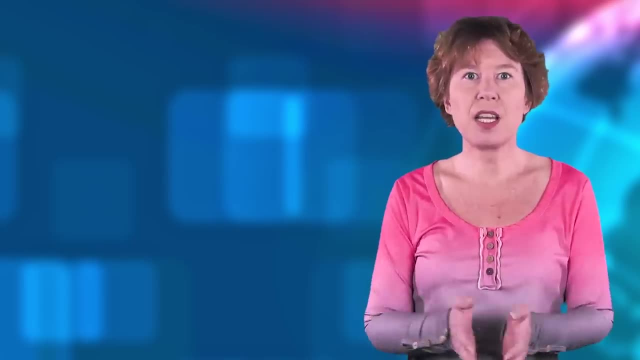 that also solves the problem, Though it isn't irrelevant to mention that most of the proofs it found were considered considerably longer than those from humans. But the significance of alpha geometry's achievement goes beyond solving geometry problems. It generally highlights AI's growing ability to reason logically, discover new knowledge. 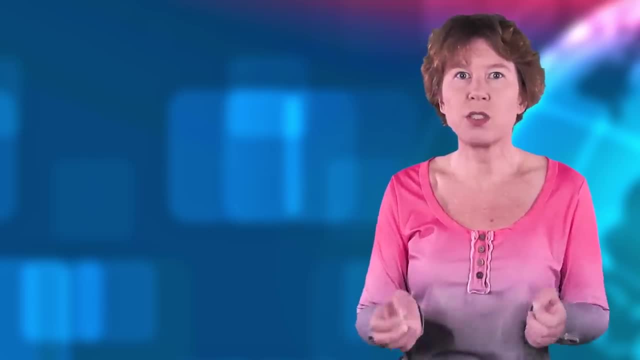 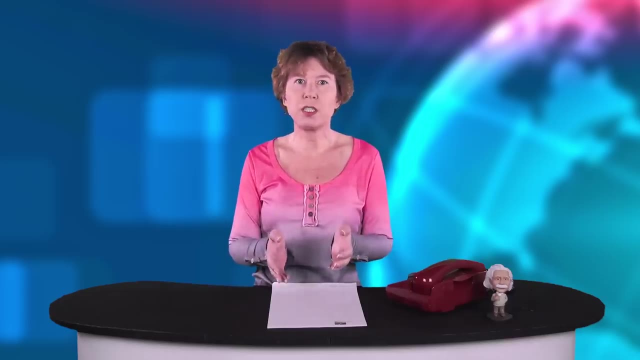 and verify solutions. And not only this, it can also explain how it arrived at a conclusion. Such a type of AI system has uses that extend beyond geometry. Not only can this achievement be generalized across various mathematical systems, but it can also be applied to other systems. 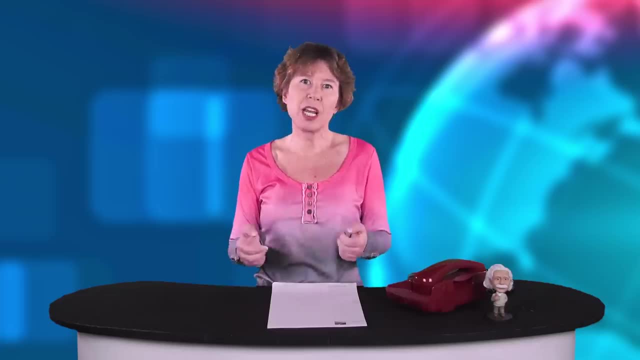 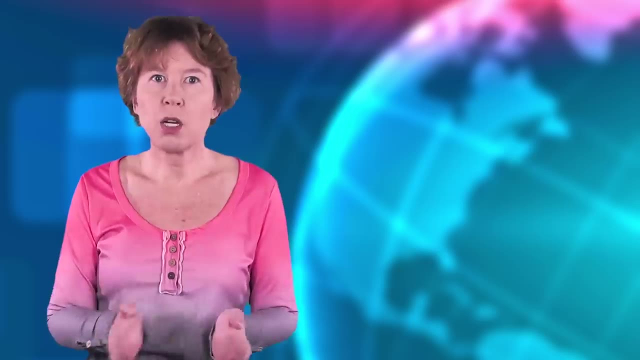 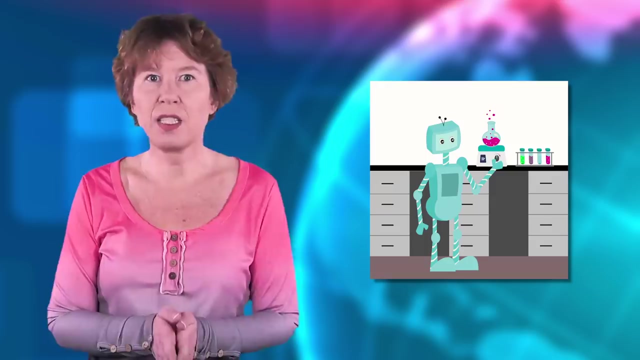 But it'll, without doubt, also come in handy in other areas where rational thinking and logical deduction is of use. Like everything. Now throw in a bunch of data in addition to the reasoning skills, and you have the perfect scientist: Unbiased, clear-headed, able to digest huge amounts of data and draw logical conclusions. 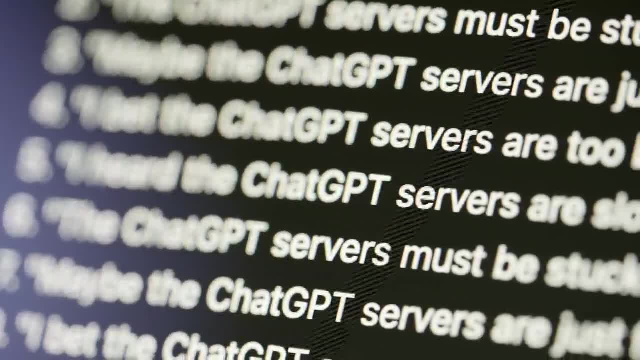 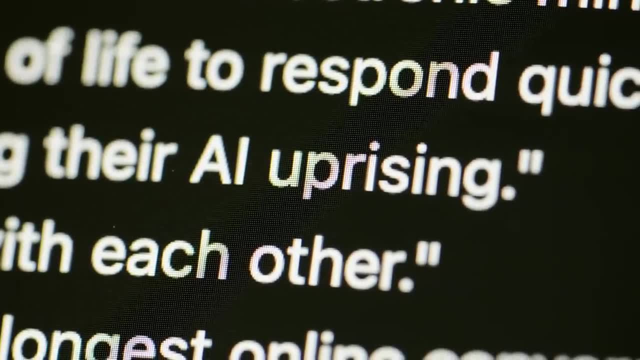 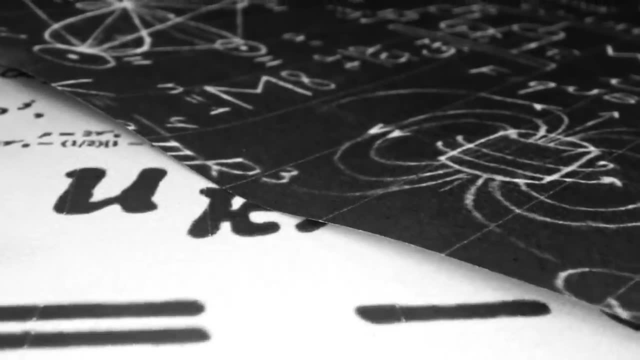 from it That alpha geometry is able to explain how it arrived at a conclusion should also help alleviate the fears of paper People who think that AI will be a black box that no human can follow. You see, the thing with mathematical proofs or arguments in general, is that it's difficult.